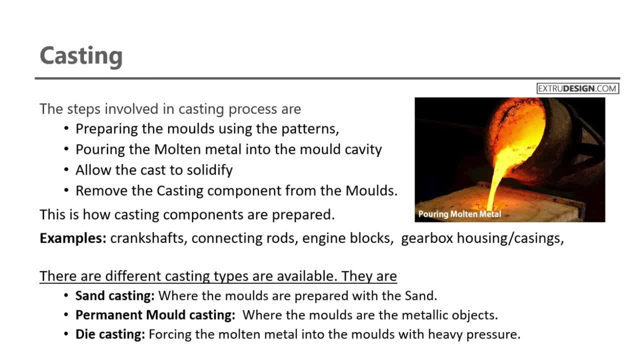 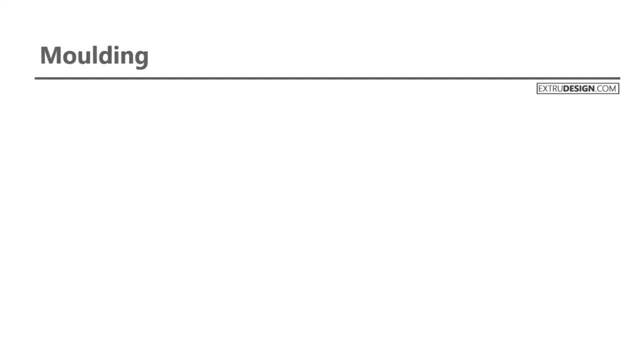 the molds are prepared with the sand, whereas permanent mold casting, where the molds are metallic objects, with the die casting forcing the molten metal into molds with heavy pressure. this is all about casting. the next one is molding. molding is the process of making objects by shaping liquid or pileable raw. 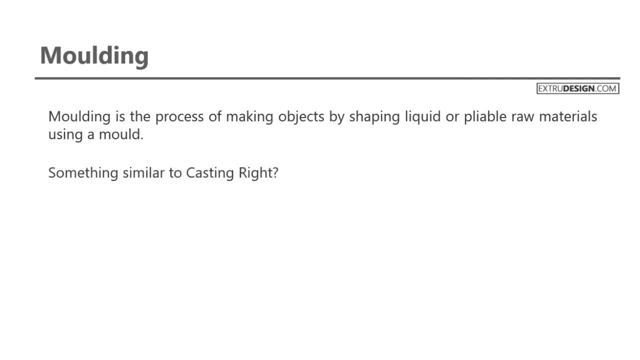 material using mold, something similar to casting, right, but really there are not same. molding is the manufacturing process of non-metallic objects when further machining is not done required, but casting refer to the metallic objects where further machining is required. this is the main difference between casting and molding. 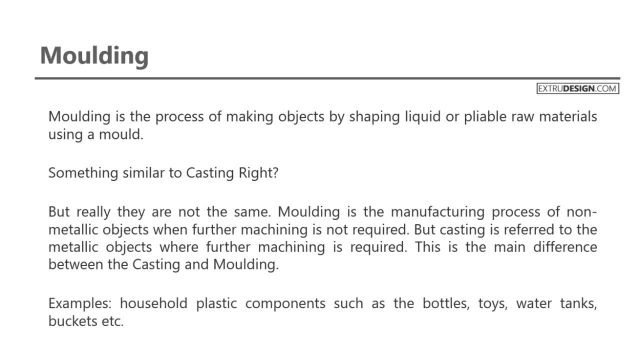 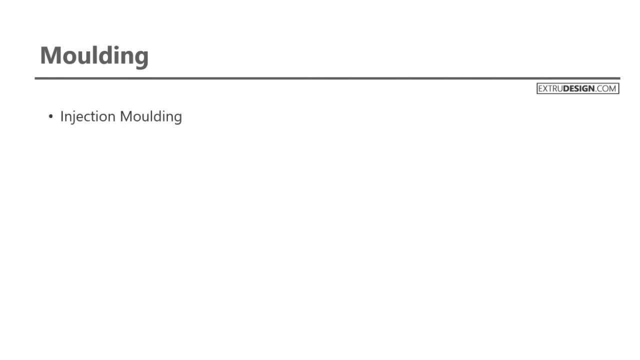 examples of molding are household plastic components such as the bottles, toys, water tanks and buckets. these all components are made from molding. there are different molding methods available. the first one is the cast molding. the cast molding is the process of making objects by shaping liquid or pileable raw. 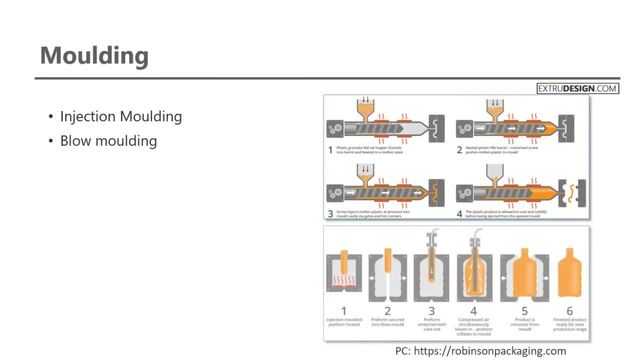 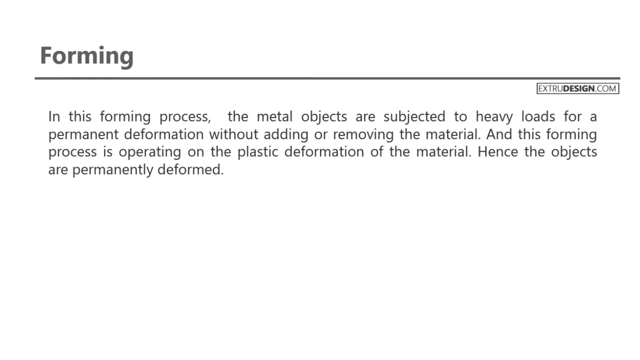 material. the first one is injection molding, blow molding, compression molding and rotational molding. these are the four different molding methods. we have discussed this molding methods in a separate video. please check the description for the video link. and the next one is forming. in this forming process, the metallic objects are subjected to heavy loads for a permanent 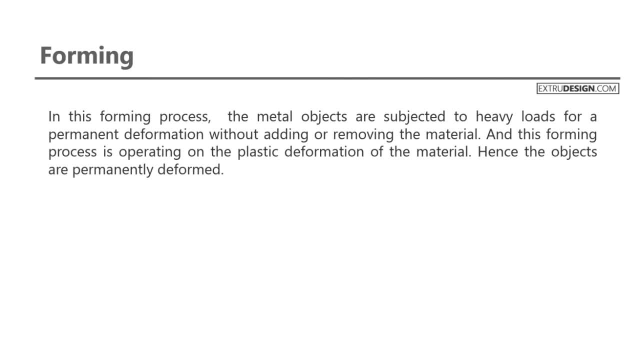 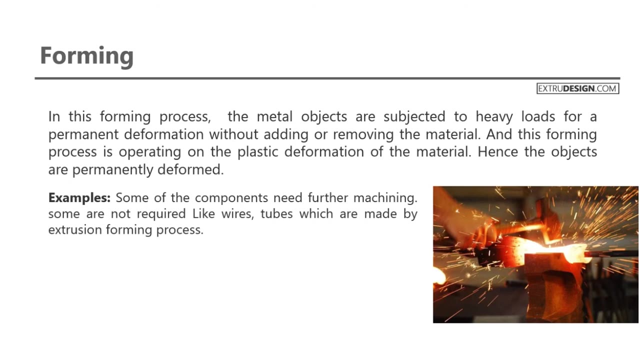 deformation without adding, are removing the metal, and this forming process is operating on the plastic deformation of material. hence the objects are permanently deformed. examples are some of the components need further machining. some are not required, like wires, tubes, which made by extrusion forming processes. the farming process has different categories based on: 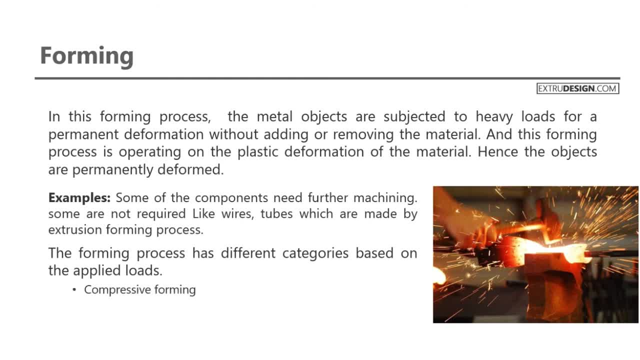 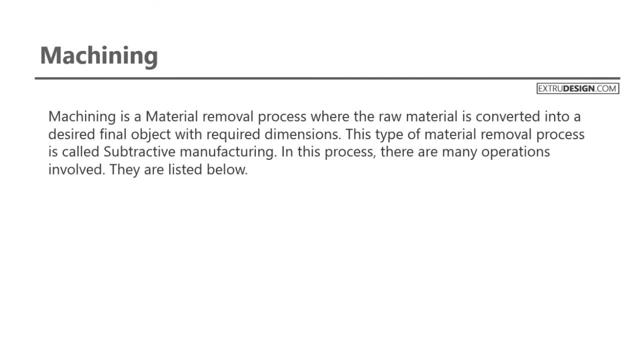 applied loads of different materials to form the material and then the materialäridirable. Those are compressive forming, tensile forming and bending and shearing. These are the different forming processes And the next one is machining. Machining is a material removal process where the raw material is converted into desired final object with required dimensions.